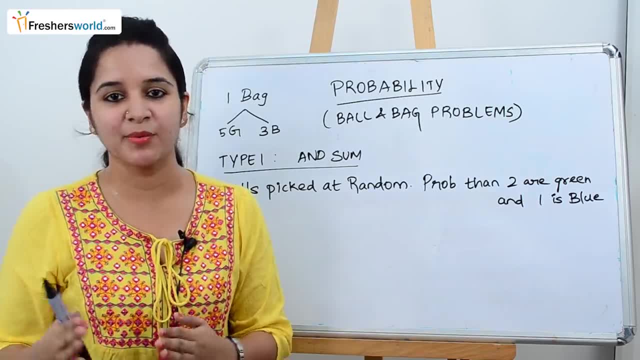 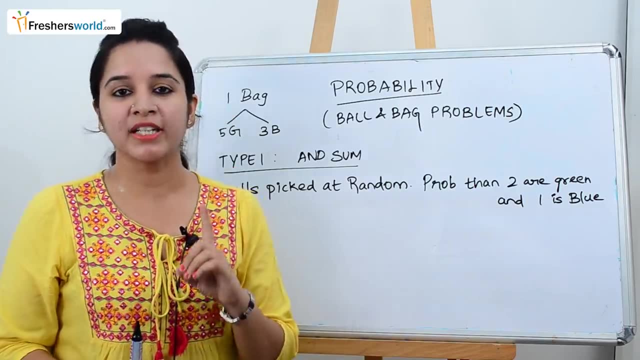 similar type of back problem for all the seven types that I'm going to discuss. A bag has five green balls and three blue balls. Let's get started with the type one. So type one sum that you can expect in a ball and back problem is and sum. So let's get started the question So. 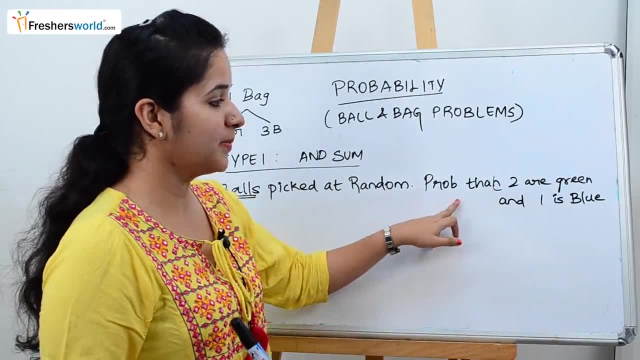 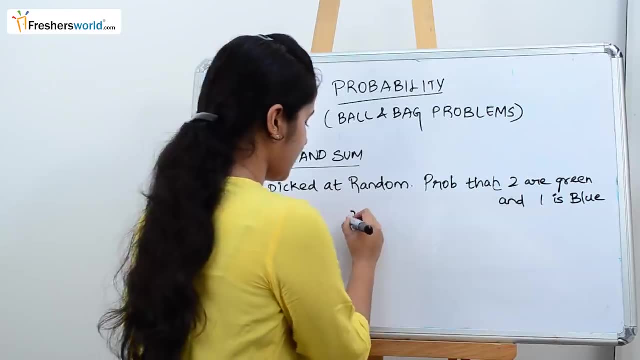 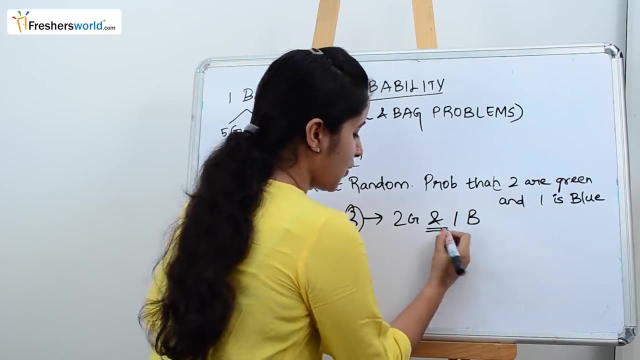 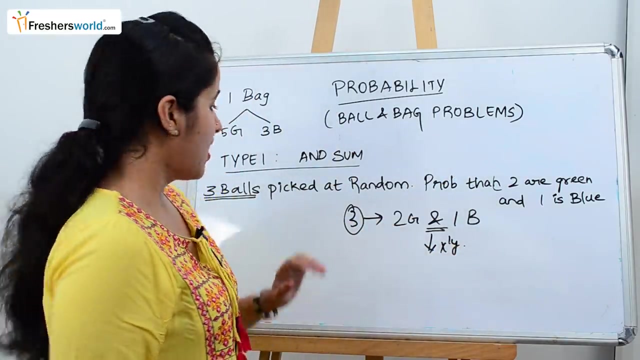 the question has three balls picked at random probability, that two are green and one is blue. Okay, so the question has total balls, is three, out of which what we need to choose two green balls. So, immediately, when you see and multiply the answer, So we are selecting three balls, So a. 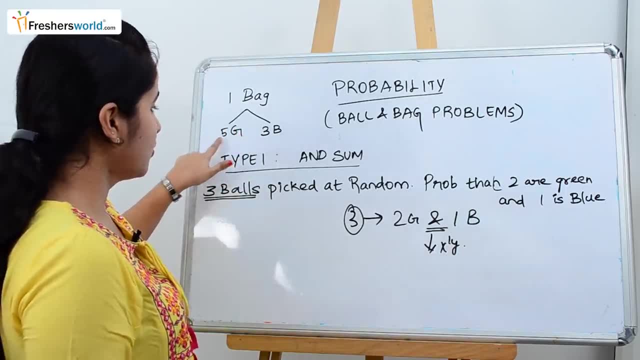 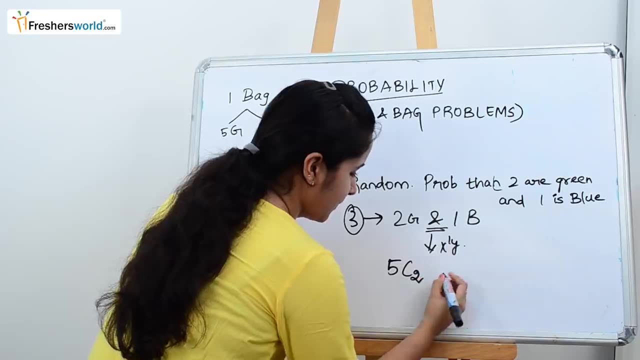 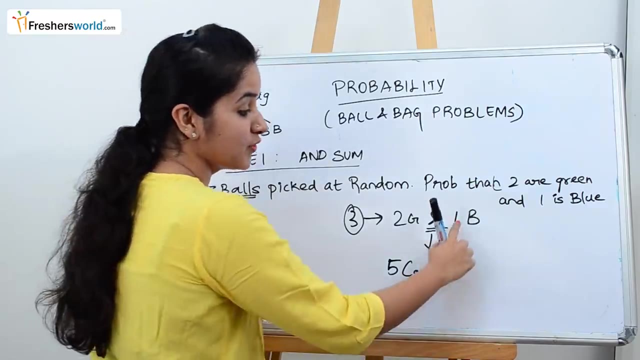 bag has five green balls and three blue balls, So total number of green balls is five, out of which we are choosing two, So five c two and as and is there, we are multiplying it. Similarly, total number of blue balls is three, out of which we are choosing one, So three c one divided by three. 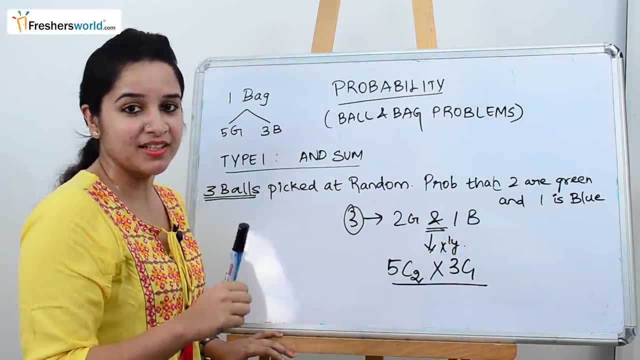 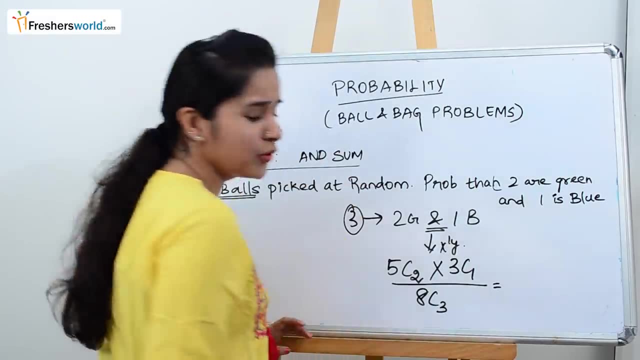 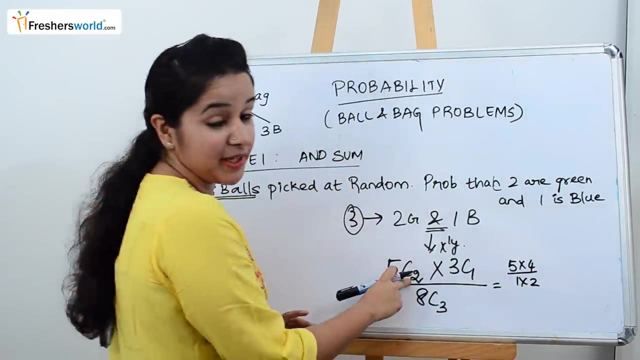 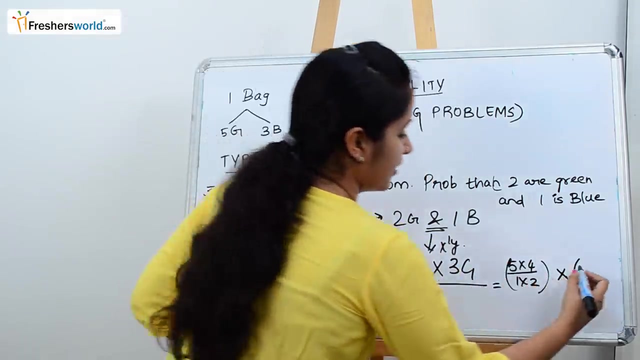 divided by what is the total number of balls? five plus three, which is eight. out of which how many balls you have to choose? three, So eight c three. If you don't know the formula, it's always simple: five into four, divided by one into two, number of times, you reduce the numerator into three c one. 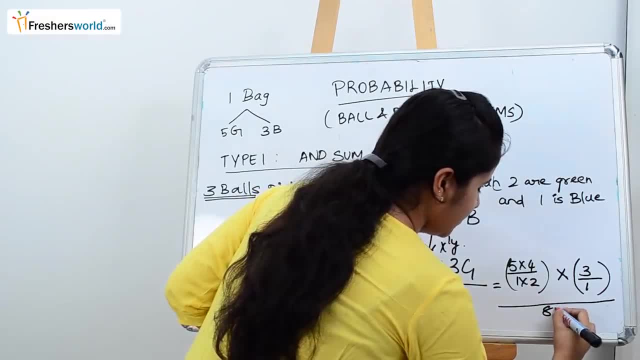 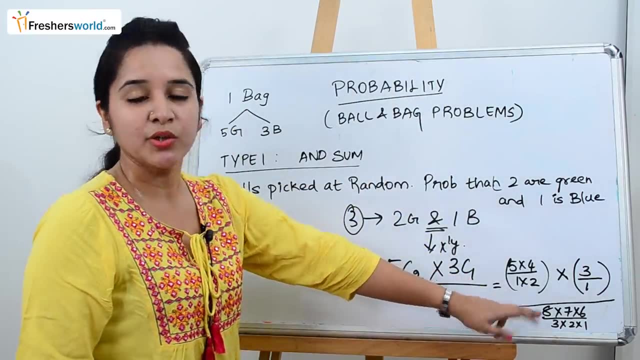 divided by eight, c three, which is eight into seven, into six. divided by three into two, into one. So if you solve it, you will get the answer. So let's get started with the type two sum. So type two is awesome. So the question that you 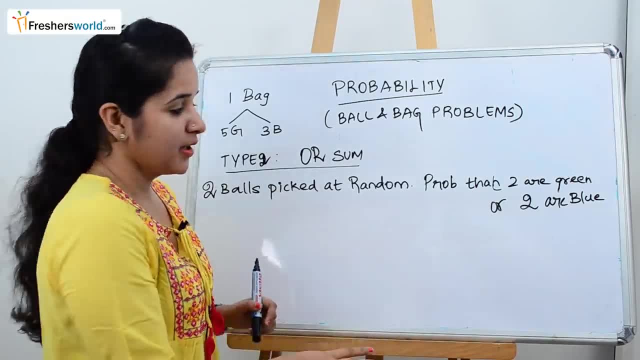 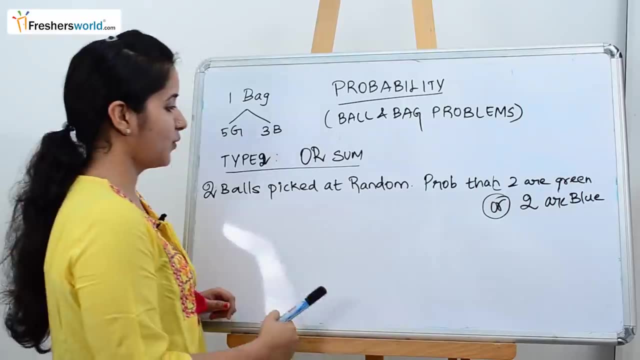 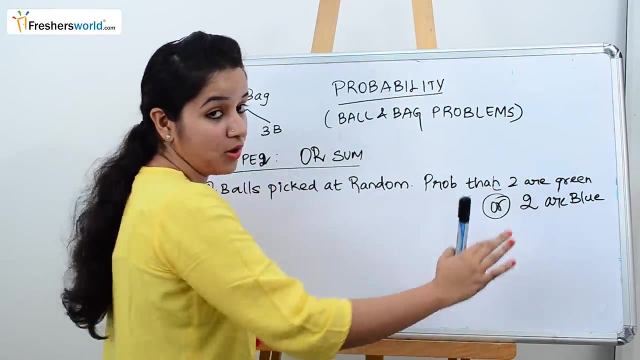 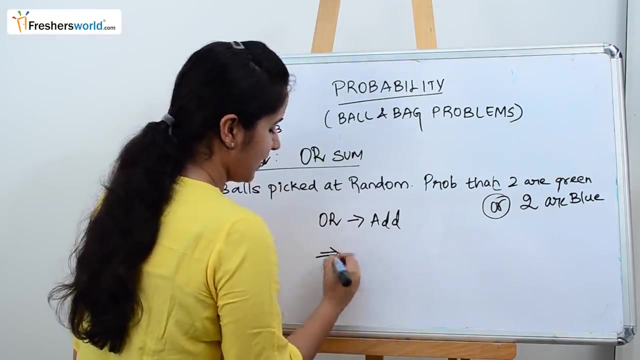 have got is two balls are picked at random probability, that two are green or two are blue. Remember the catch word. So the overall question is: a bag has five green and three blue balls, out of which either two are green or two are blue, Immediately when you find the word or add it, So the answer will come as you have to. 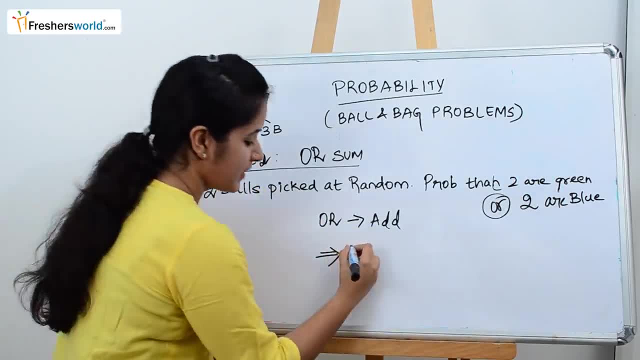 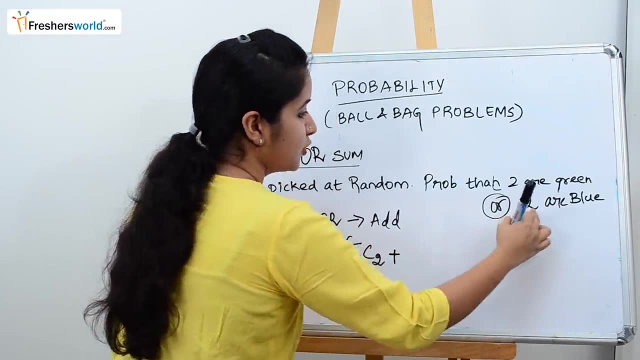 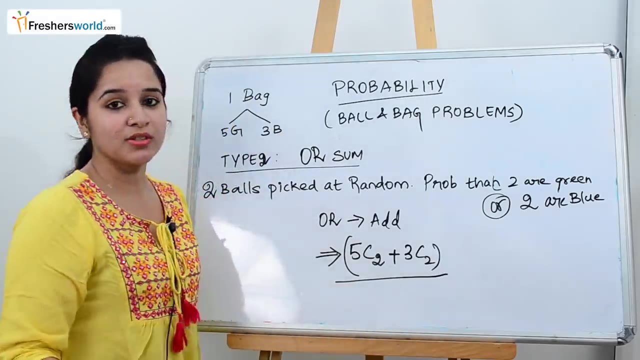 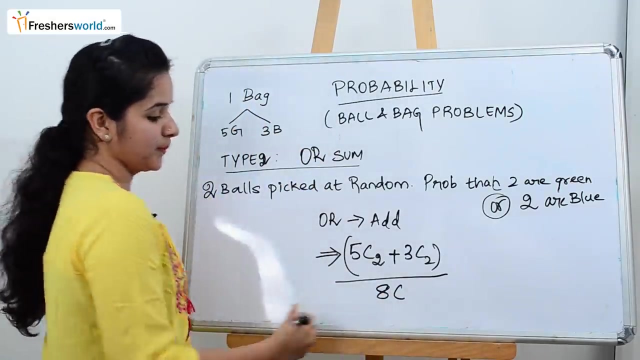 choose two green balls out of five. green balls: five, see two. So you have all here. So what do you do? you add: two are blue out of three blue balls. So three c 2 divided by what is the total number of balls, five plus 3, which is 8.. See how many balls you have to choose: 2. 8C2.. Let's just simplify it: 5 into 4. 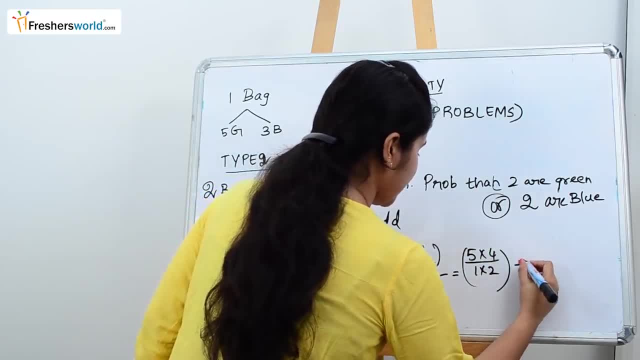 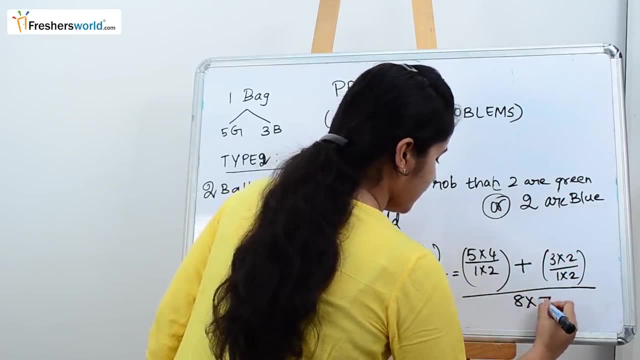 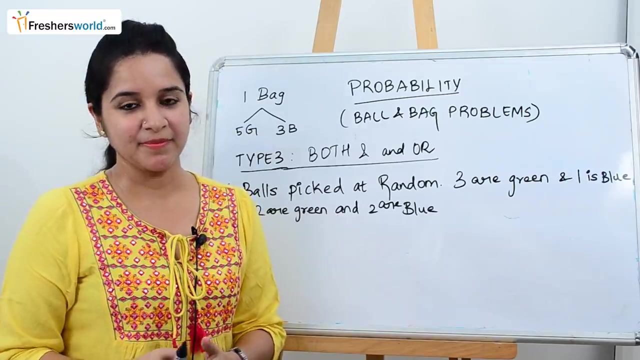 divided by 1 into 2 plus 3 into 2. divided by 1 into 2. divided by 8 into 7, by 2 into 1.. Once you simplify it, you get the answer for this question. Let's go to the third type of sum. So this is a. 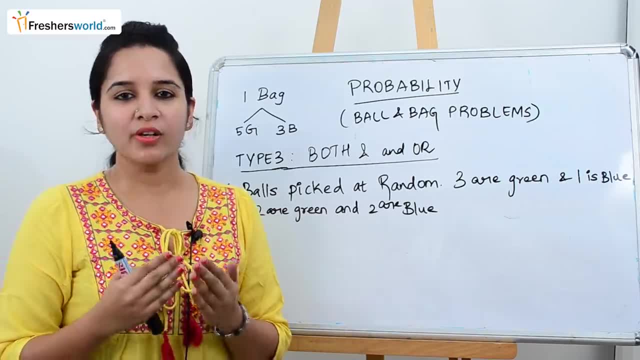 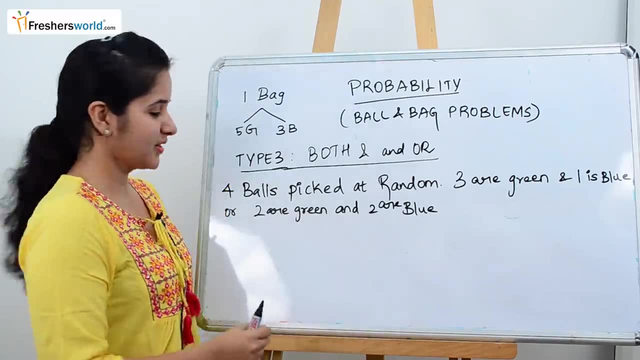 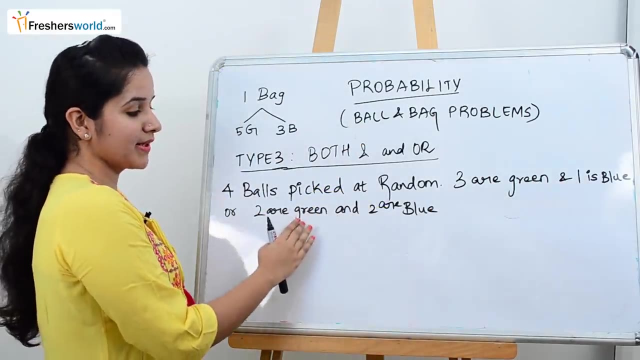 combination of AND as well as OR problem. So you already dealt with the AND and OR problem separately. Now it's a combination of both. Let's get started. So the question is: 4 balls picked at random, 3 are green and 1 is blue, or 2 are green and 2 are blue. So the catch here is: 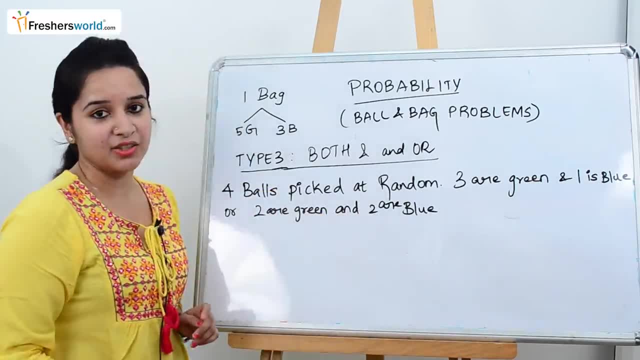 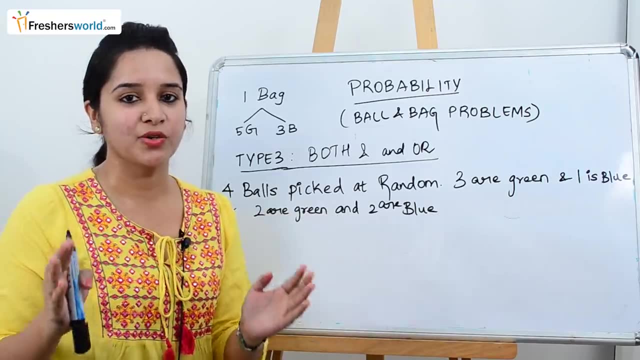 people get confused with AND OR and AND here in the question. So while you are seeing the question itself, you put a bracket in the question and confirm where you are going to multiply and where you are going to add. So 3 are green and 1 is blue. bracket OR will be in. 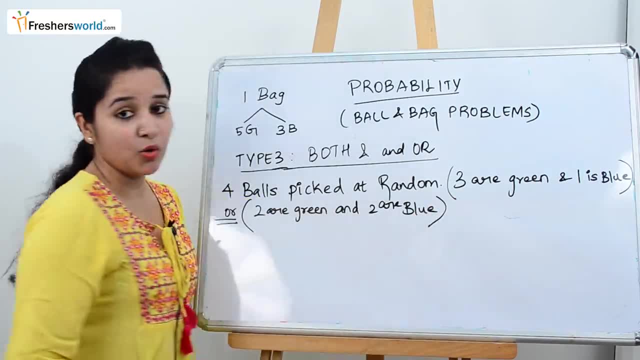 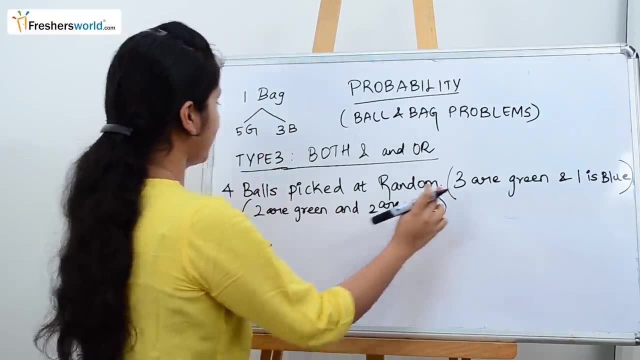 between. 2 are green and 2 are blue. Now we can easily write the answer. So for first, for this, 3 are green. How much from 3 you are taking? So there are 5 green balls, So 5, 3, 3.. If you see, 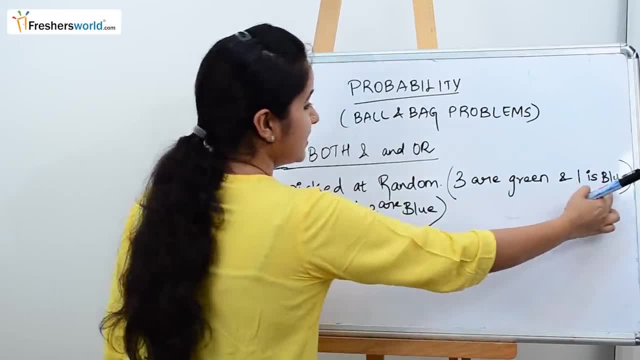 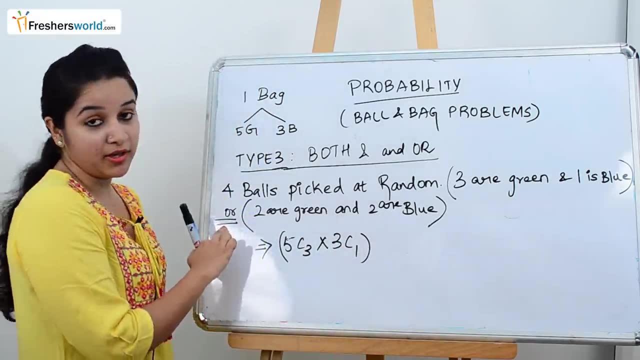 AND what do you do? You multiply. So 1 is blue. Out of how many balls? 3 balls, So 3, C1.. Put a bracket Now. OR OR means addition, So you add it here. So 2 are green and 2 are. 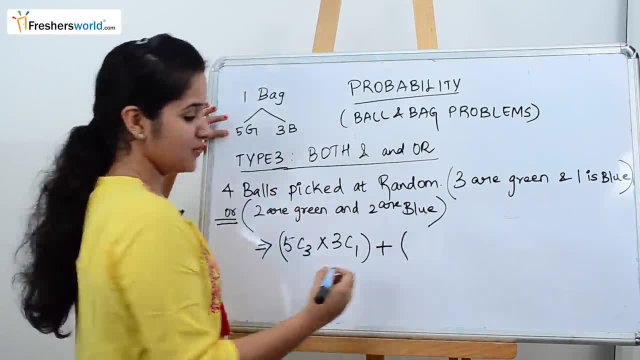 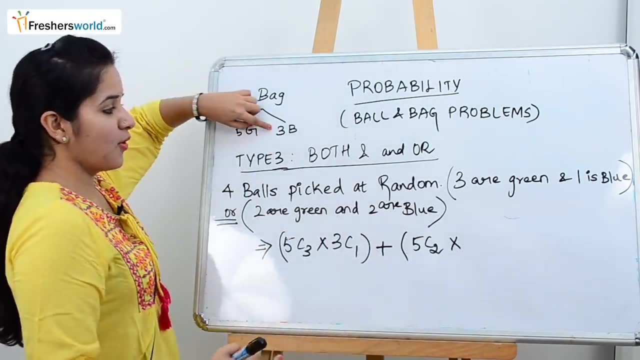 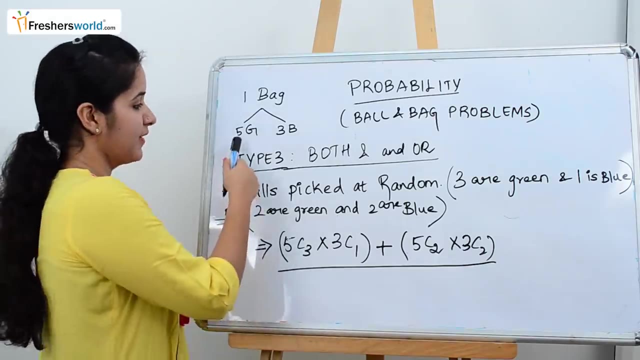 blue, So 2 out of 5 balls we are taking. So 5, C2 multiply because we have- AND here and 2 are blue- 3 balls we are taking 2.. So 3, C2 divided by how many balls we have, 5 plus 3, 8 balls out.